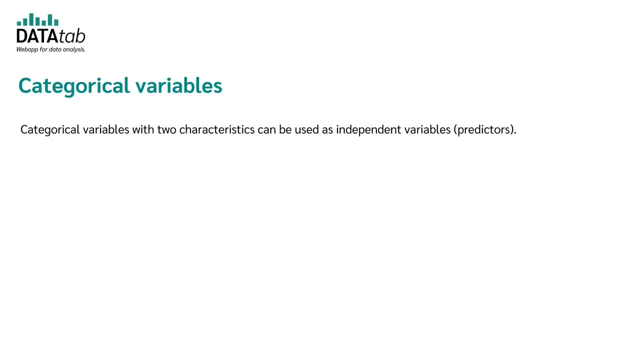 as independent variables, also called predictors. Categorical variables are either nominal or ordinal variables. Categorical variables with two expressions are also called dichotomous. An example would be gender, with the categories male and female. Let's say, you coded female as. 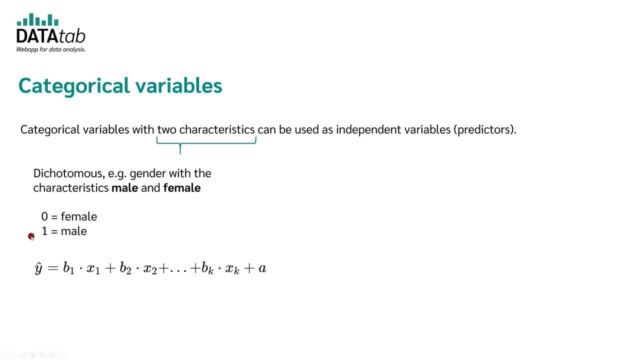 zero and male as one. In that case female would be the reference category. If we now look at the regression equation and say the variable x1 is gender, then b1 is the regression coefficient for gender. So the question now is how can we interpret b1?? We said that zero is female and one is male. So we just 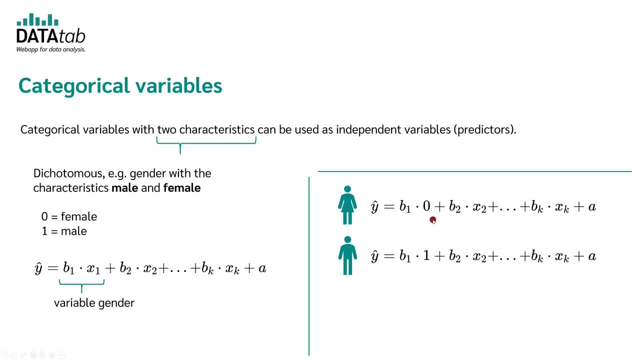 put that in, Then we have zero times b1 for a female person and one for a male. So we have zero times b1 for a female person and one for a male person, And one for a male person, And one for a female person, And one for a male person And one for a female person. 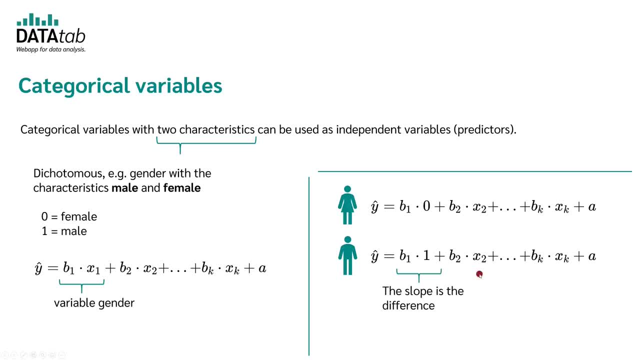 one time B1 for a male person. Accordingly, B1 indicates the difference between male and female. Let's say, in this example we want to predict the income of a person, so Y would be our income. If a person is male, this person earns more by the amount of B1 than a woman. Therefore, 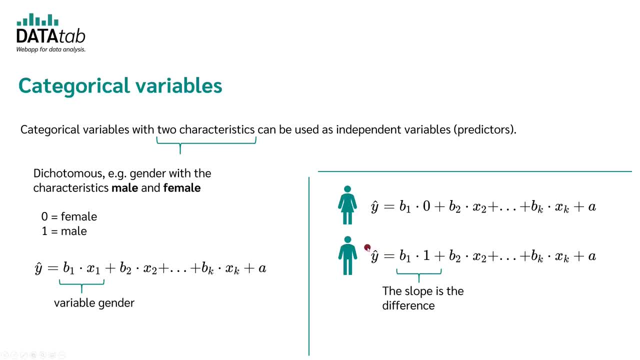 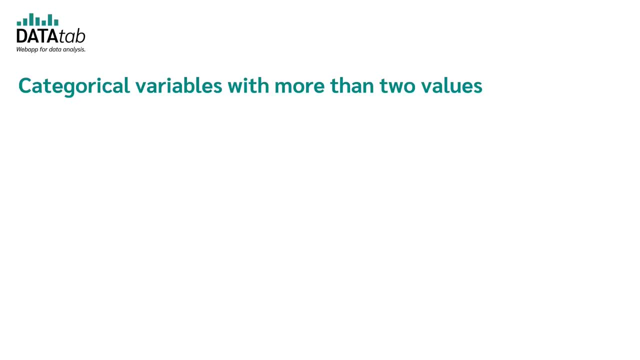 B1 is the salary difference between men and women. Now we have discussed how to handle variables with two characteristics. Now let's take a look at what we do when we have a variable with more than two characteristics. Let's look at an example. In this example, we want to predict. 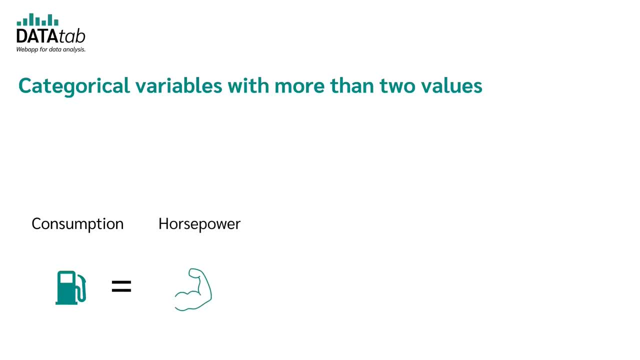 the fuel consumption of a car based on its horsepower and the vehicle type, And let's say there are only three. We have three vehicle types: sedan, sports car and family van. Thus, we have a variable vehicle type with more than two characteristics. In a regression, however, we can only consider: 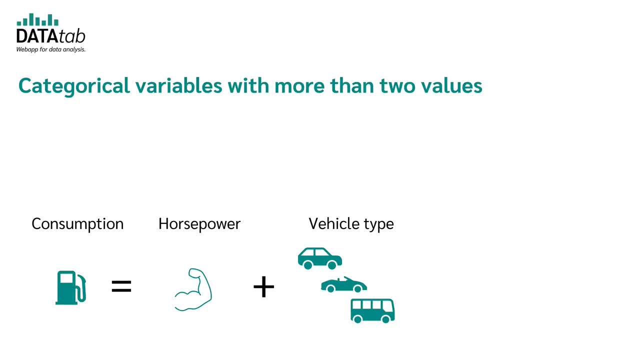 categorical variables with two characteristics. Therefore, the question now is: what should we do In order to use categorical variables with more than two characteristics in a regression model? we have to create a variable with more than two characteristics, So we have to create a variable. 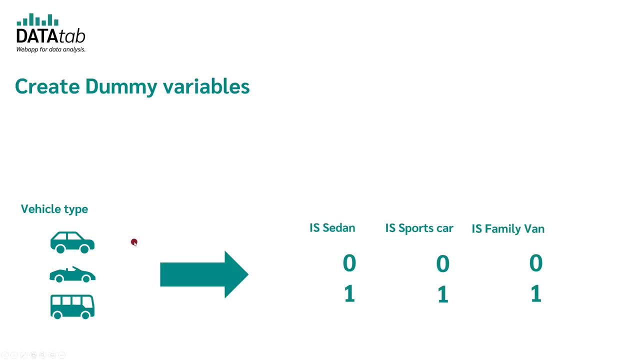 with more than two characteristics. This means that we simply create three new variables. Each new variable has two characteristics. These characteristics are 0 and 1, or yes and no. So in our example we have our vehicle type with the characteristics sedan, sports car. 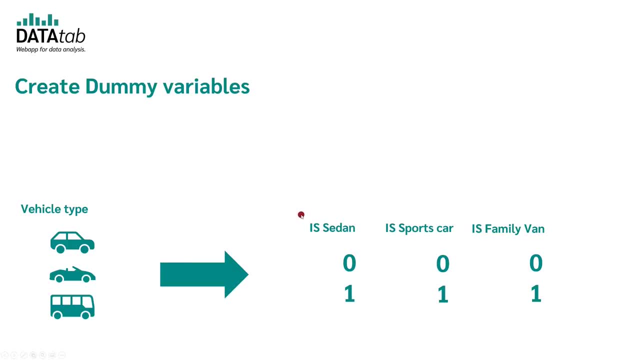 and family van. Now we create one new variable out of these characteristics. This means that we have three new variables out of each characteristic. So this means we create one variable which says: is it a sedan? yes or no, Is it a sports car- yes or no. And finally, is it a family? 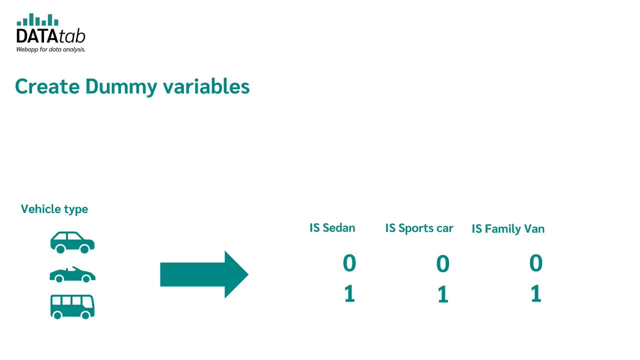 van yes or no. So before we had one variable. Now we have three variables, which are dichotomous and therefore have only two characteristics, And these three new variables can be used in our regression model now. So what does that mean for your data preparation now? 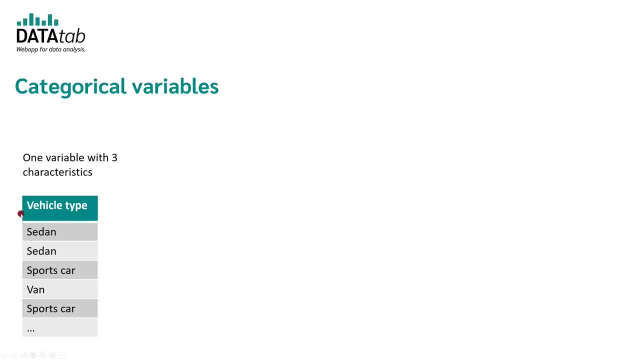 You originally have one column with the vehicle type, where the individual vehicles from your sample are listed. The first is a sedan, the second is also a sedan, the third is a sports car, and so on and so forth. Out of this table, you create your new three variables now. So the question is: what is? 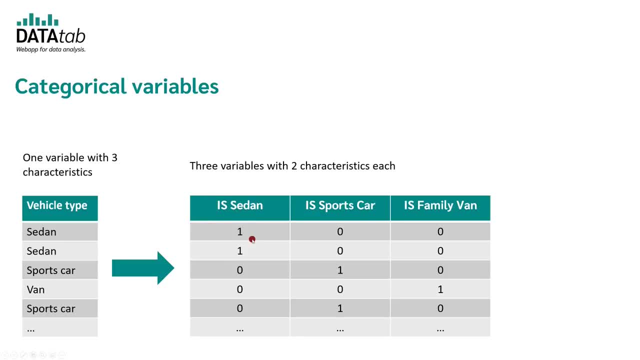 the first car Is it a sedan, So you put a one here and a zero for the other cars, Because it is not a sports car and it is not a family van. The second car is also a sedan, so we'll put a one here, And the third one is a sports car, so we'll put a one in the. 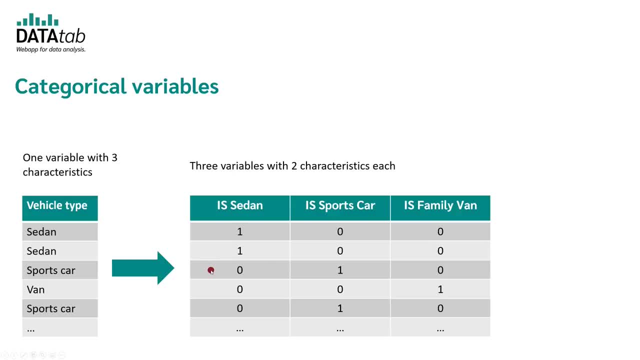 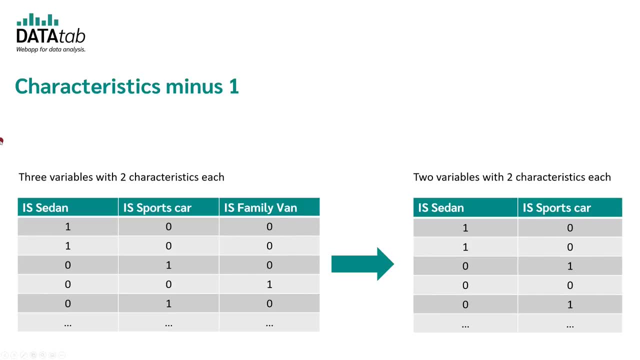 column sports car- and a zero for the other car types. So with this procedure we finally formed our dummy variables. Now there is still one important thing to note: The number of dummy variables formed is always the number of characteristics minus one. With these two variables we have the